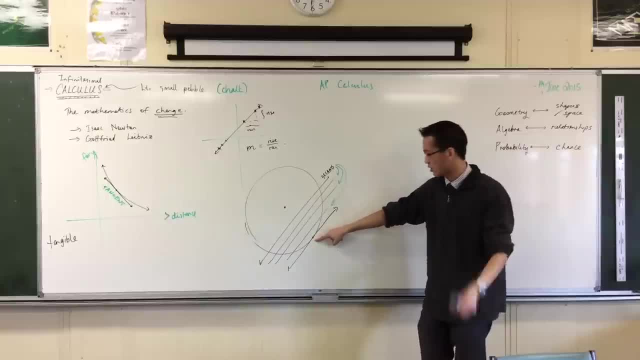 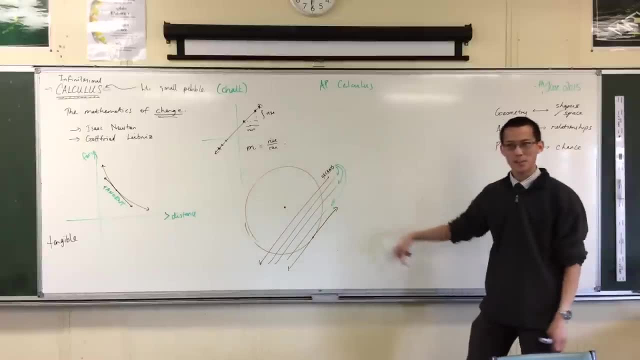 It's not actually a chord, it's just a single point. That's why it's actually zero. So what Newton wanted to do was take this problem apart by thinking of it like this, As one of these problems. he thought: what if? what? if I could, I can understand the behavior of this secant. 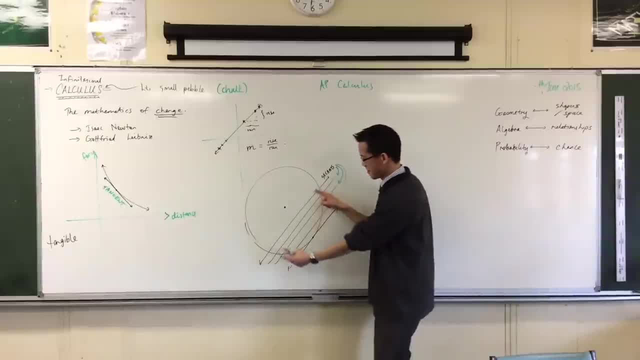 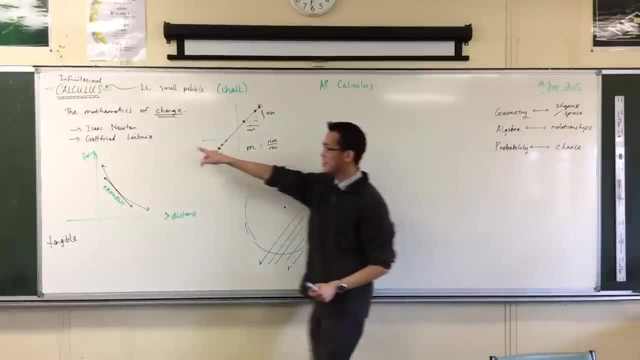 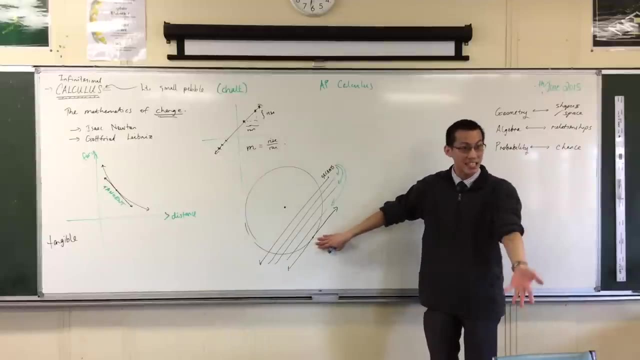 What if I could imagine it as it approaches a chord of length zero, If it approaches a chord of length zero. So both of these guys, both of these guys said: I need some language. I need some language to talk about things that approach something which, you know, I can't actually get to. 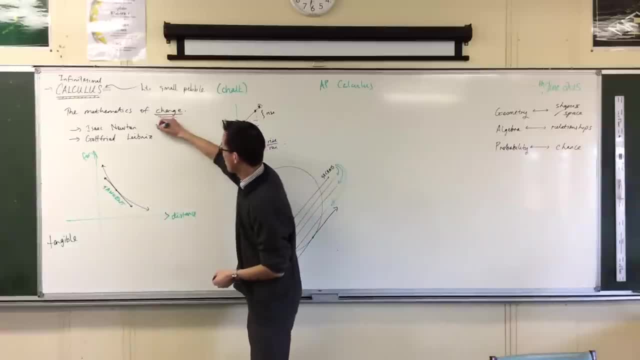 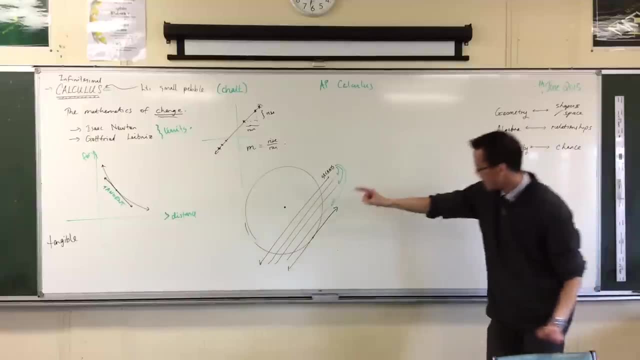 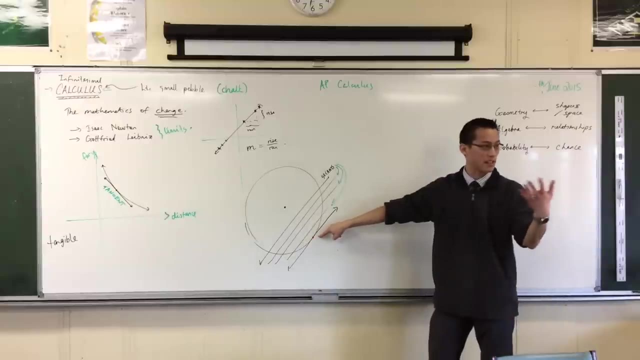 but I can still do the calculations on it. So they said let's talk about limits. They introduced this notation to something getting closer and closer and closer until you're actually there. Right, You make conclusions off of things that you know so that you can draw some information about something you don't know. 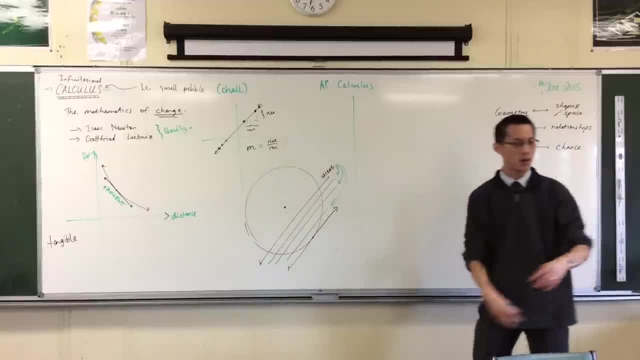 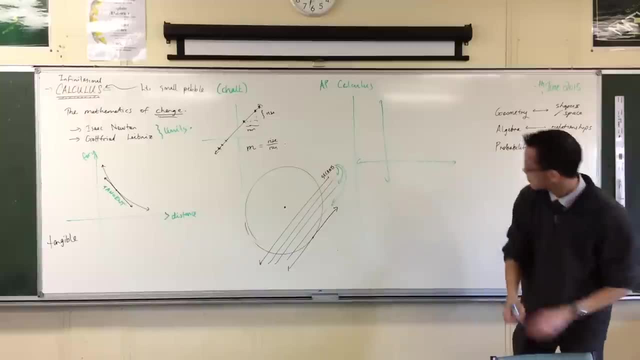 Okay, So now here's where the rubber hits the road. Draw for me a new set of axes. Let's just go first quadrant. that's all you need Now. draw for me a curve. Draw for me a curve, And let's call this some function of x. 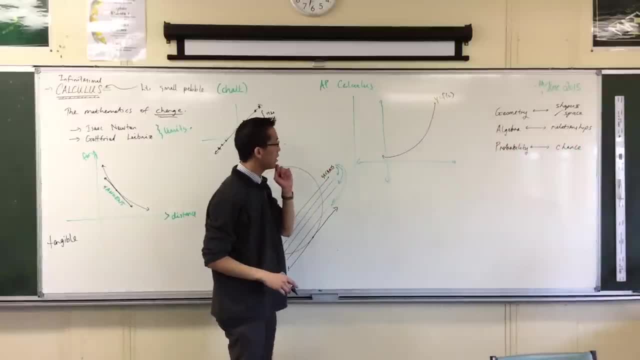 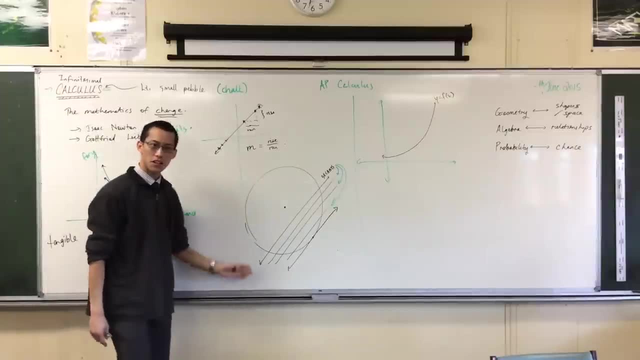 Some function of x. Okay. Now, if what I'm after is the gradient of a tangent, gradient of a tangent, okay, what I'm going to start thinking about is the gradient of a secant, and think about what happens to that as it gets closer and closer to becoming a tangent. 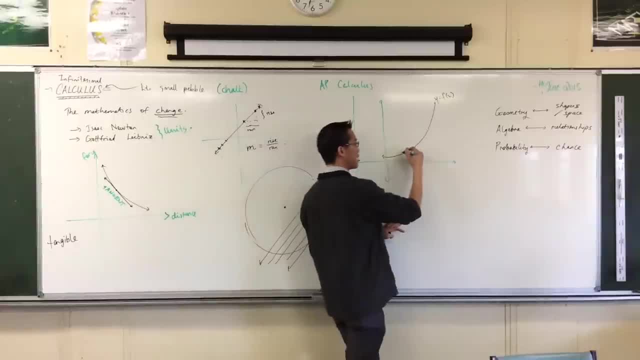 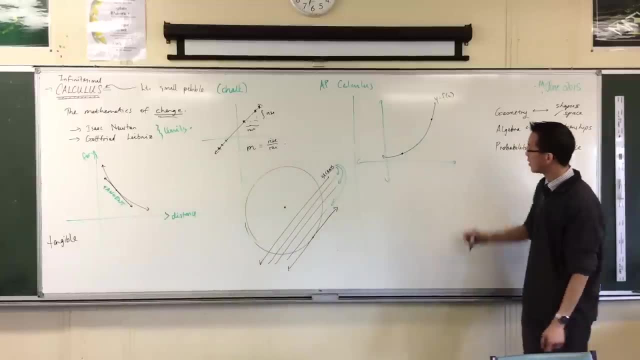 Right, So in order to get a secant- that's not hard- You just pick any two points you like, like here and here. Okay, And what you see like if the actual point I'm after is like somewhere in the middle here. 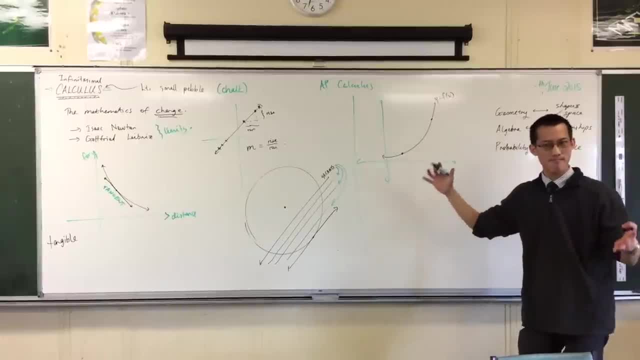 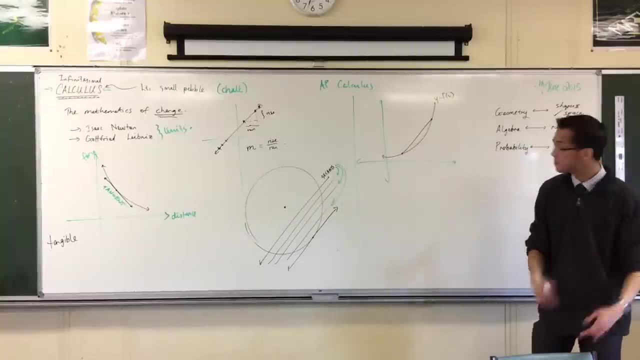 Okay, If you were to draw that tangent, it's actually not that far off in terms of its gradient compared to this secant Right Like I'm in the right ballpark. Yeah, So I've got these two points. I've got these two points. 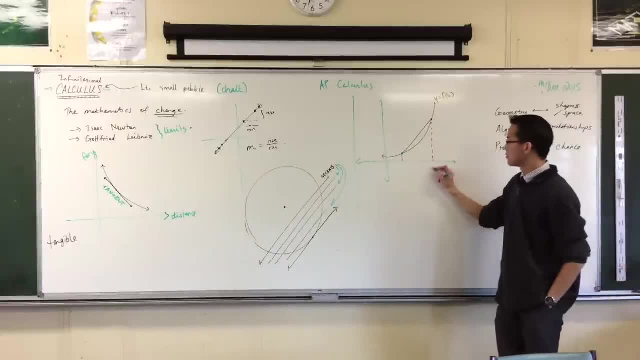 Let's get some values on this. Alright, If I imagine this is some x coordinate- Who cares what it is, I'll just call it x. I want it to be anywhere that I like. I want to be able to input some value there. 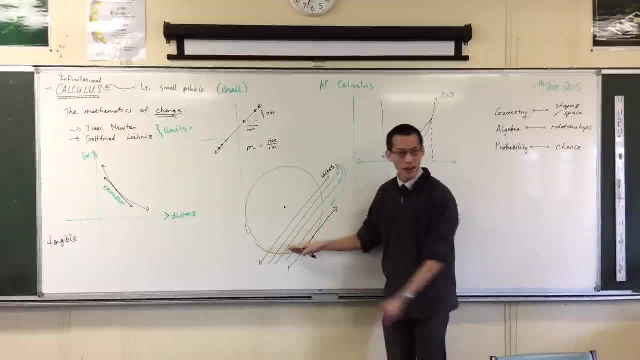 Okay, And what I'll do is I'll think about going from that point and going a bit further Right, Going like a distance of, say, they call it h. Okay, You can think that h is kind of like for height, but that's not the best description because it's further. 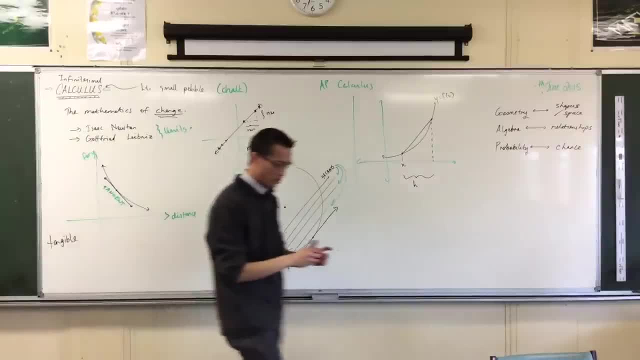 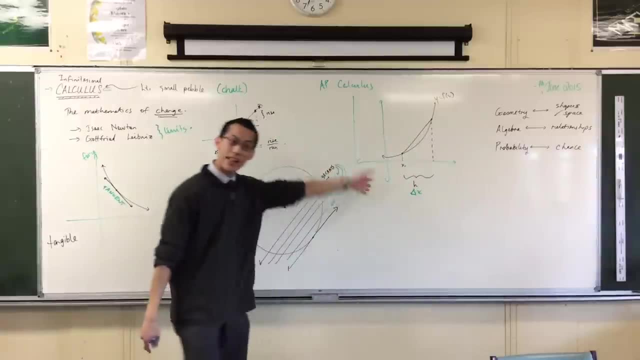 Anyway, h is the convention. There are other conventions as well. Sometimes you'll see it called delta x. We'll talk about y in a second. Now, if that little distance there- it's just a small distance- is h, then what's the coordinate of this point over here? 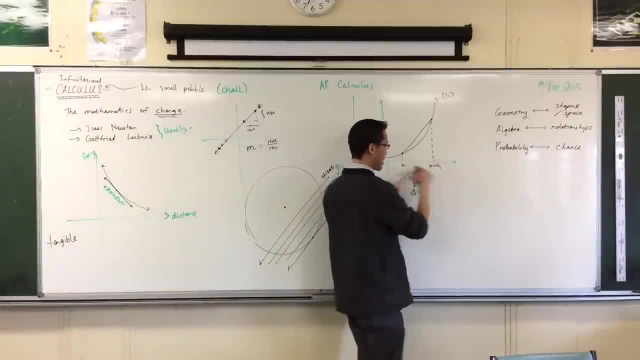 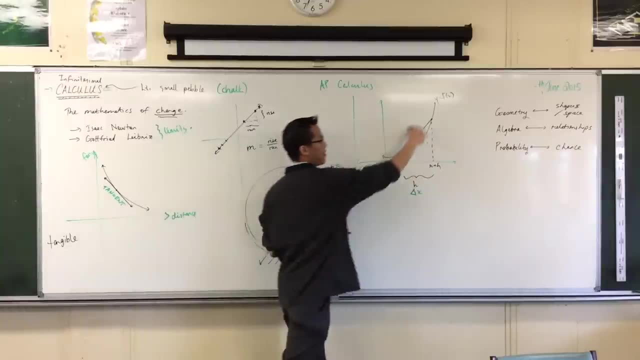 Oh, I should say the x coordinate. It's x plus h, right, It's just that plus that. That gets you over there. Okay, So now if I want to work out the gradient of this secant here, right? 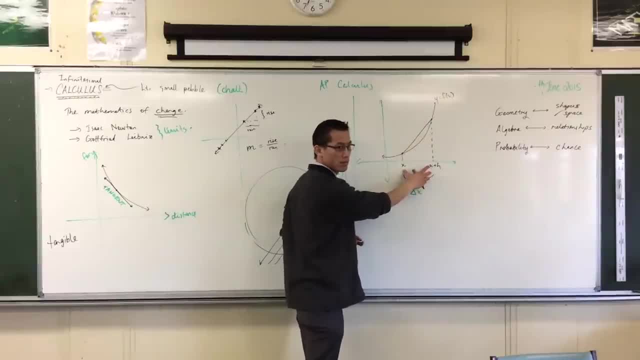 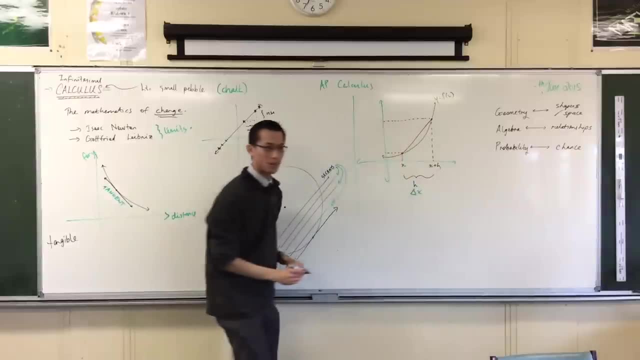 The gradient of the secant. I've got x coordinates. I'm going to need y coordinates, aren't I Right? Let's come over to here and here. Okay, Now, I don't know what this function is. It could be anything. 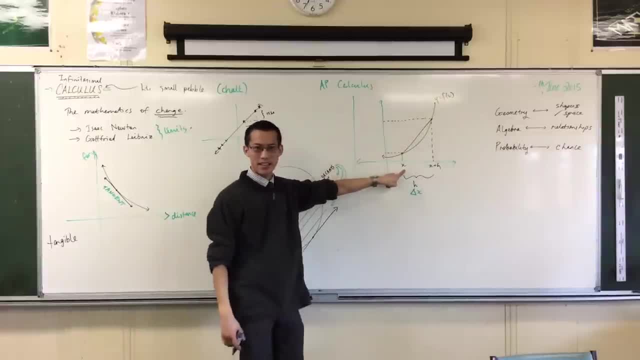 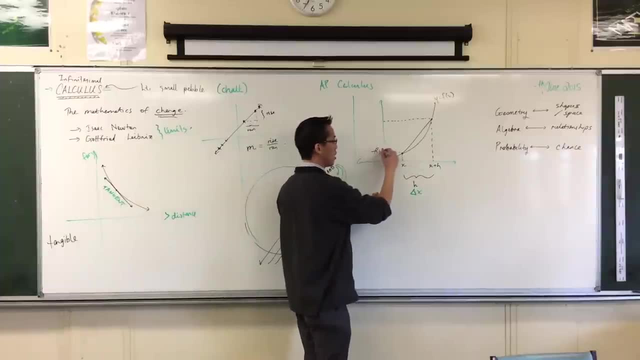 It's f of x, Right. So if this x coordinate is x, just x, right, What am I going to be up here? f of x, f of x, Good. So, for example, if this were x squared right. 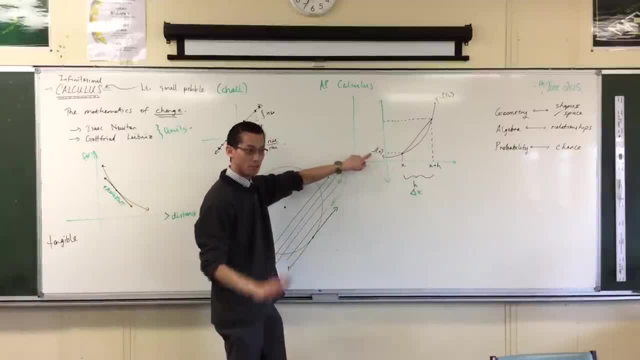 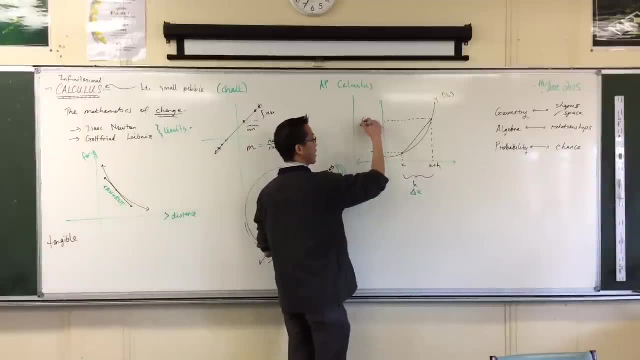 y equals x squared, then that would be x and this would be x squared Right. Simple. Now, this is x plus h, so my corresponding y value over here will be f of x plus h, Whatever f happens to be, Okay. 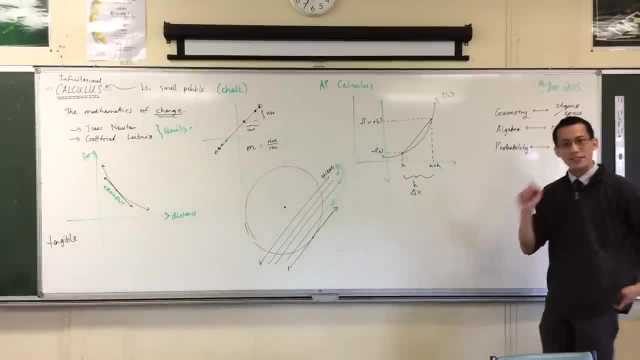 So now, what have I got here? What have I got? I've got. what I'm working out is the gradient of the secant Right, The gradient of this guy here, Okay, And it's literally just rise over run. 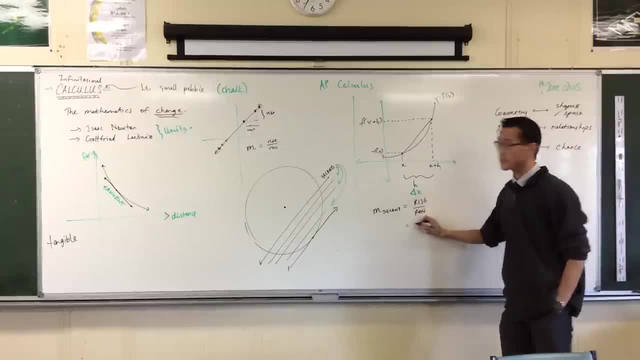 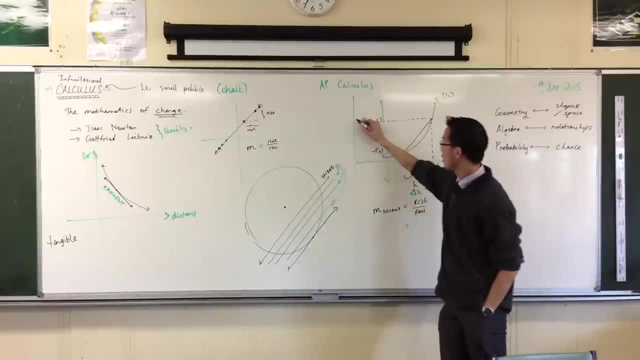 It's just rise over run, Okay. So what's my rise? Okay, It's the distance between these two key points, these two y values, Is it not Okay? What is that distance f of x plus h? Good, 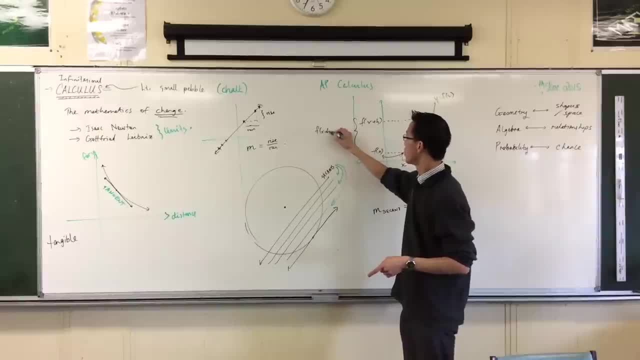 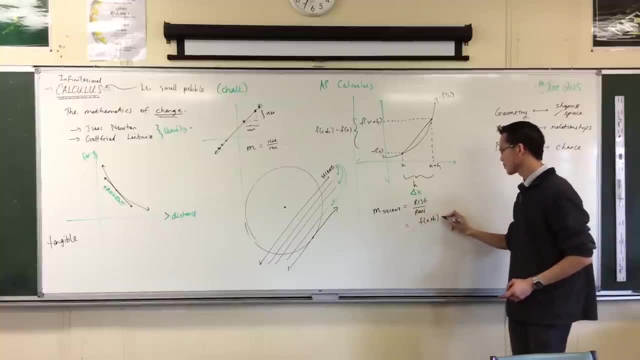 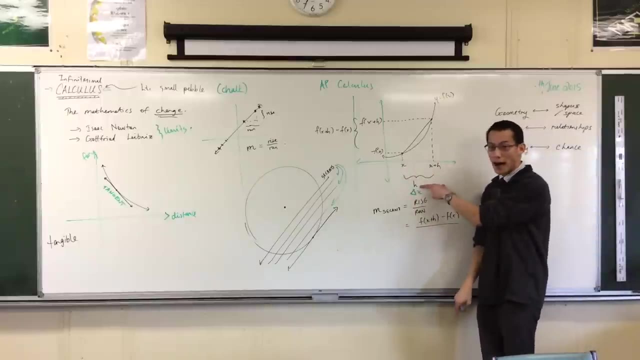 This, take away this. Yeah, That's all. that's all. that vertical distance is Okay, So rise. I've got that. Okay, Now run is the horizontal distance that I'm going. that corresponds to that Which, of course, I've defined as just h. 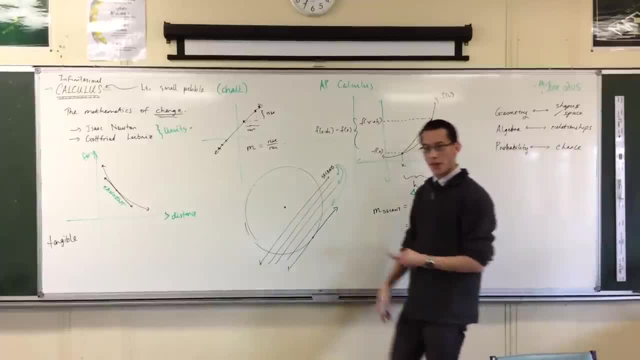 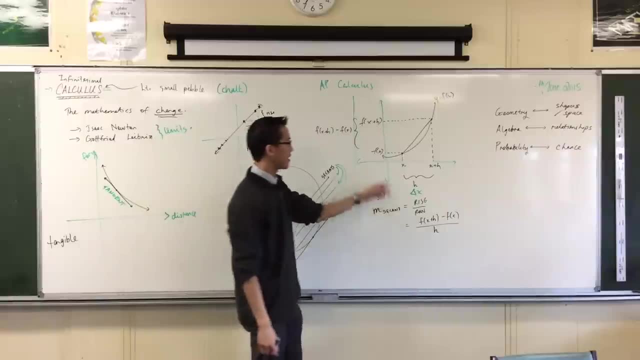 Right, It's just h. So if I have some value of x, whatever you like, Okay. And I have some function, you define it to be whatever you like, Okay. So h will give me the gradient of a secant. that's anywhere you want. 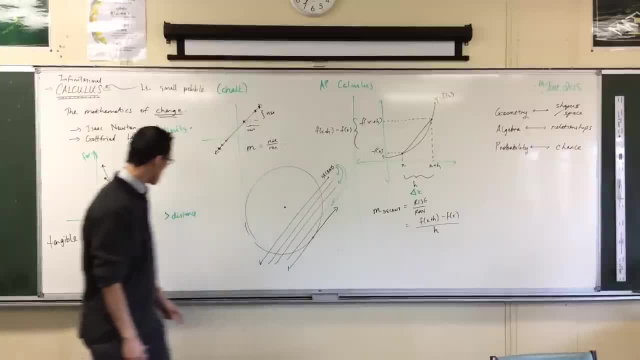 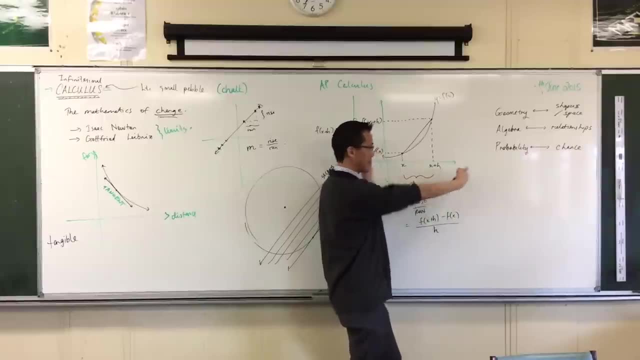 Okay, But I don't want a secant really, What I really want is at a single point where this distance in here I don't want it to be this big gaping gap in here. Okay, I want it to close in. 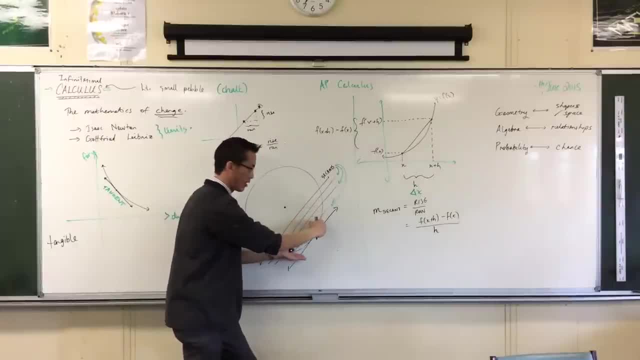 I want it to come together, just like these guys are coming together, Right. So what I want is this guy here h. I want it to get very, very, very small. Does that make sense? Now, I already have language for this. 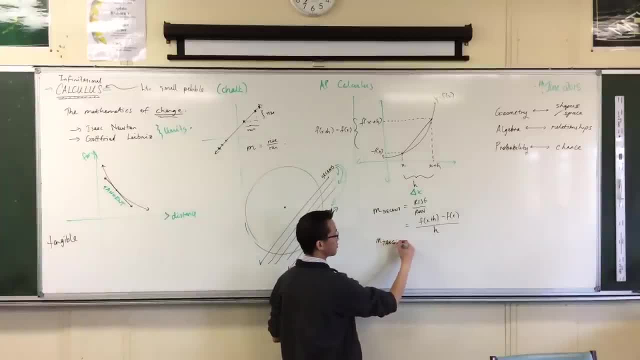 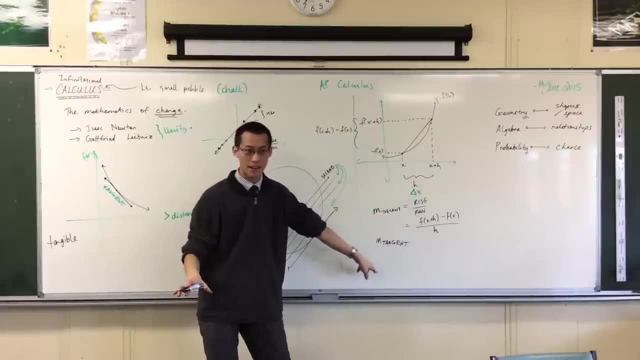 Right, When it becomes zero, I'm going to get not a secant. not a secant, but a tangent. Do you agree with that? Right, That's what I want. What I want is for h to be zero. Now, h can't really be zero. 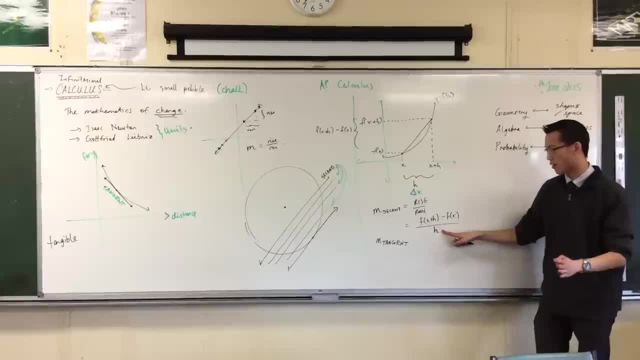 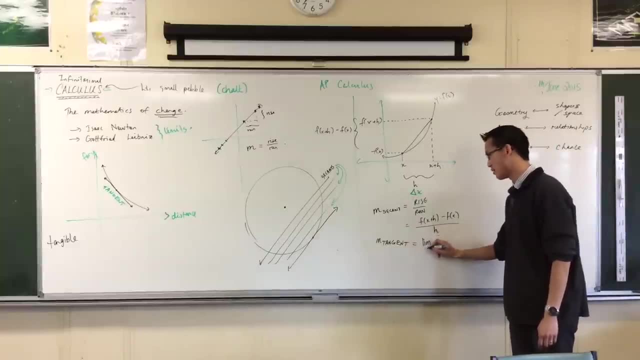 Because, look, I have to divide by h, It can't really be zero. But I can think about what happens as I get closer to zero. I just have to say: tell me What the limit is. Right, Tell me what the limit is. 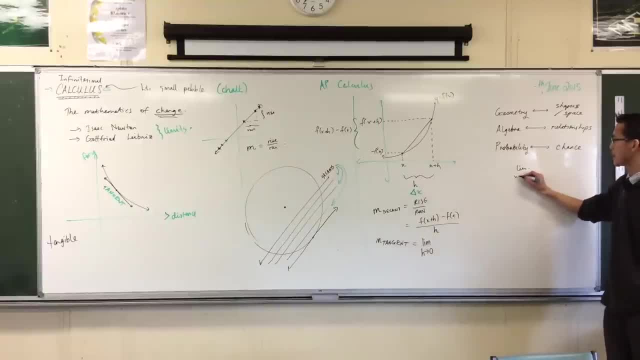 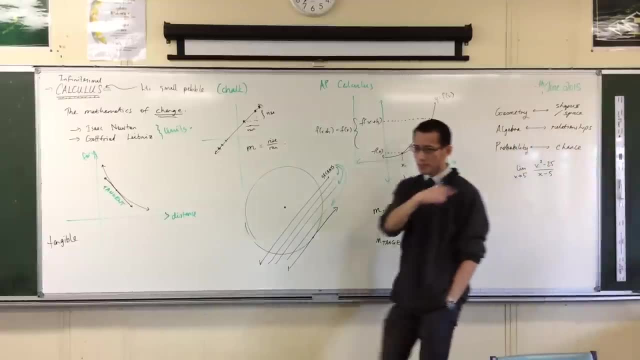 Just like we looked at before. If I gave you a trivial example: Okay, We looked at evaluating limits like that. Okay, Now that function there that I've put over here, it's got a hole at five, Doesn't it? 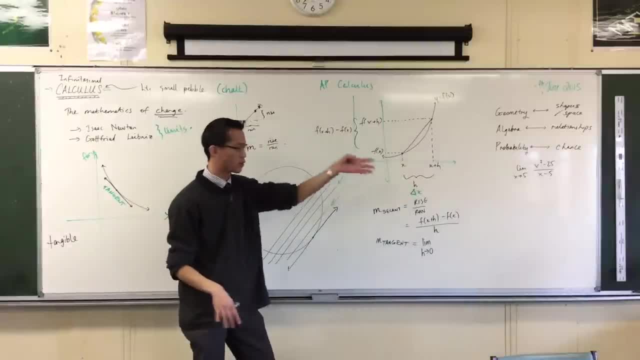 You can't equal five because it's on the denominator. So x equals five is not going to work, Okay, So what I'm going to do is I just have to say: well, that top thing, what can you do to that top thing? 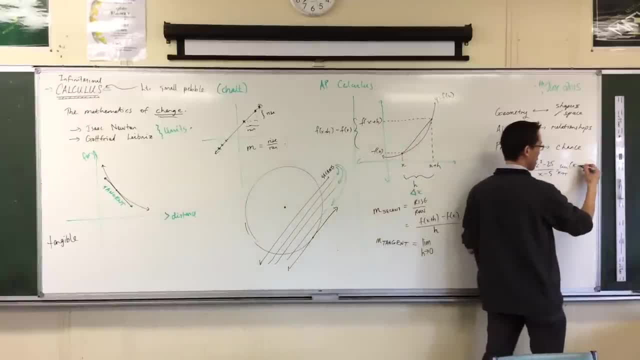 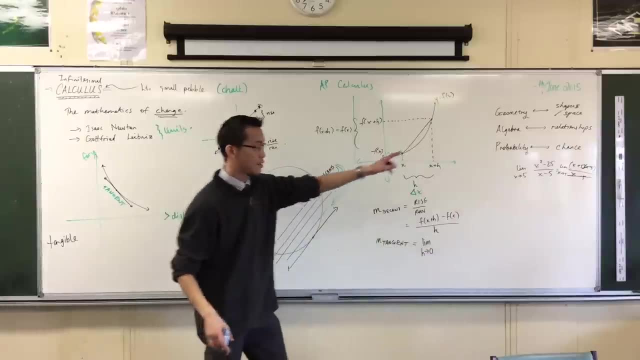 I can factorize it. It's the difference of squares, Right? So it's going to be x plus five, x minus five, And because of that our denominator goes: No problem, Okay. So at that point I can say: oh, that thing. 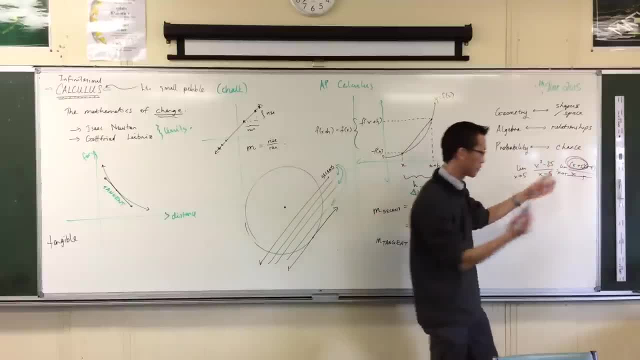 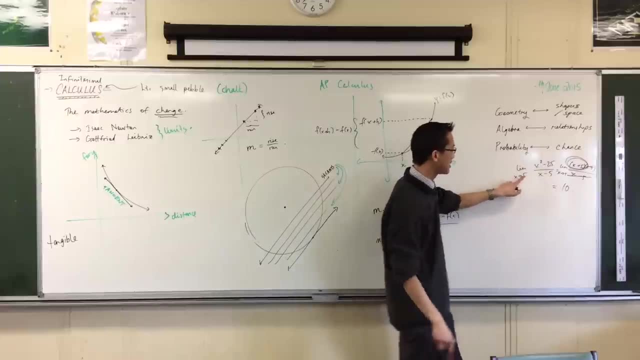 That thing That approaches five And I can actually put in five. So of course it's just going to be ten, Right? So even though this original thing I can't put five in, I can see what happens as it. 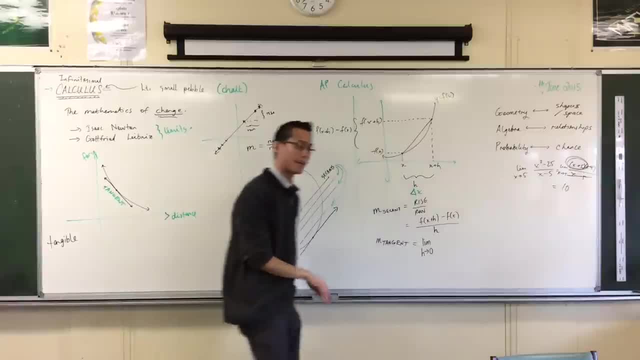 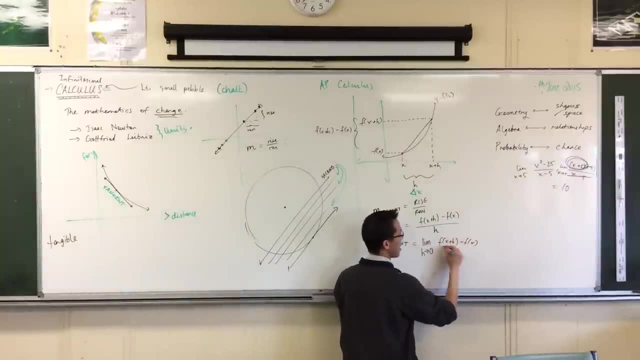 approaches five, It's going to go there. Okay, From above and below. you can go ahead and try it out. Okay, So here I can't put in zero, but I can think about what happens as I get ever closer to. 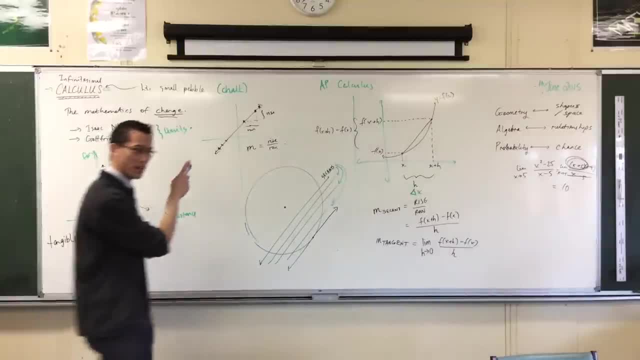 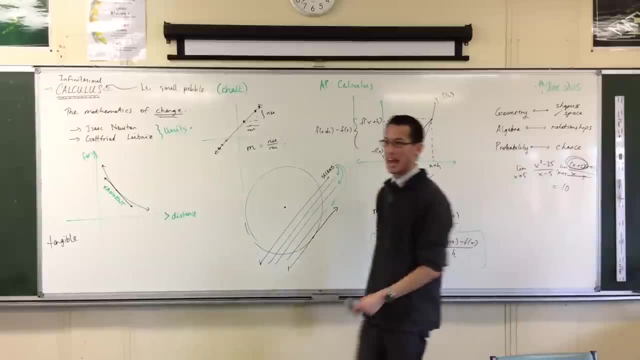 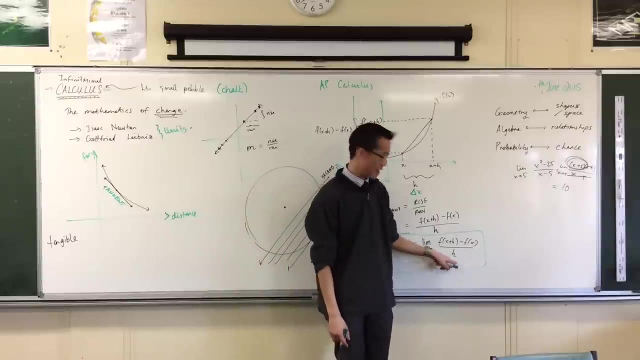 it. Okay. So this thing here, this guy, is a big deal. Okay, This was Leibniz's and Newton's big watershed moment. They're like I can't work out by just putting in zero Right At least into this, which is what it is by definition: rise over run. 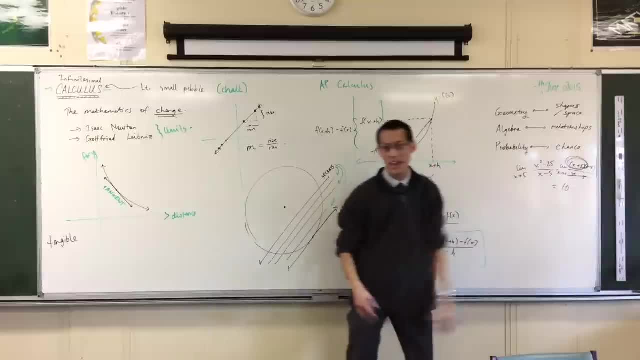 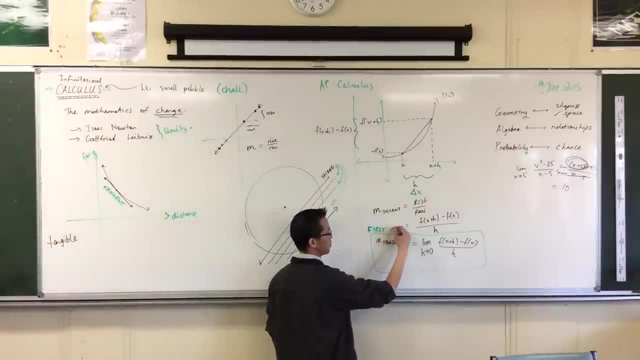 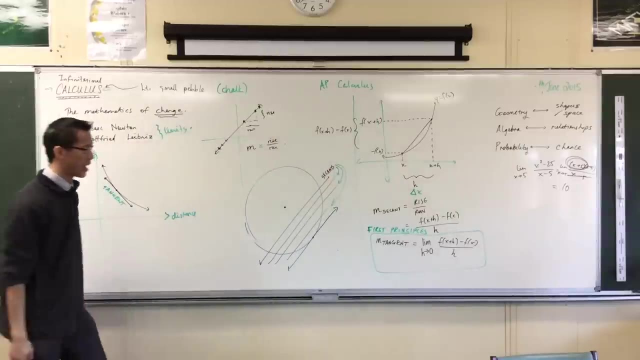 But I can still do maths with it. I can still do maths with it, even if I can't actually put zero in. This is what we call the first principles of calculus. The first principles of calculus. What are we actually working out? 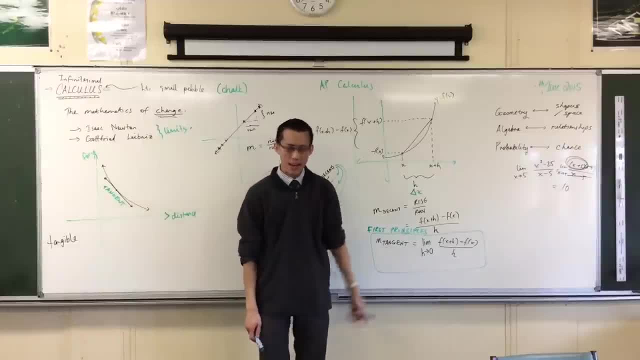 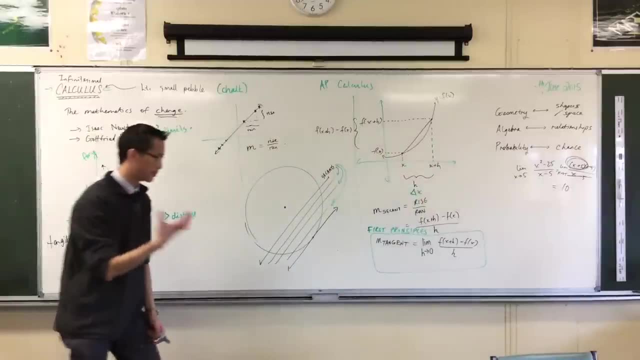 We're working out the gradient of the tangent, Okay, But this started to get a bit awkward in terms of, like, talking about all this stuff. So they introduced Newton's law, So they introduced new language and they introduced new notation. Okay, 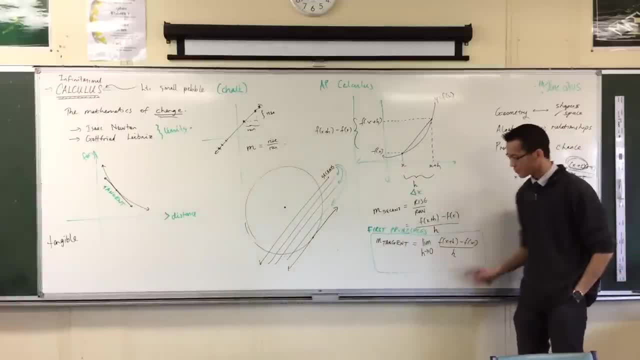 So the new language they introduced was- they called this thing right, Like I could get it at a particular point. I could get it at a particular point, But I could get it at any point. I like Right, And it's going to change all the way. 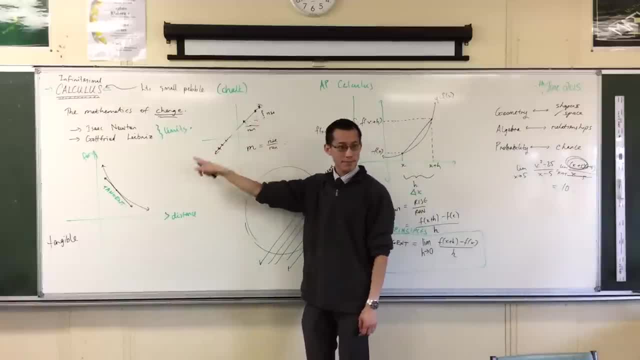 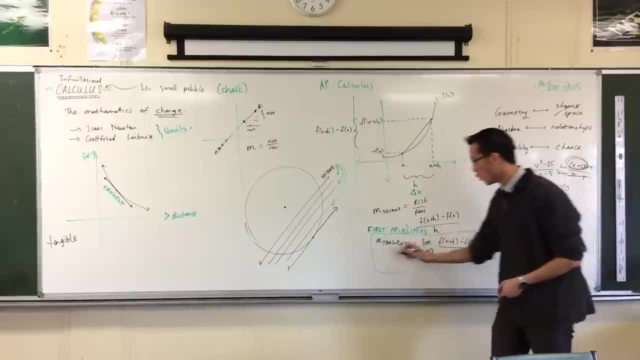 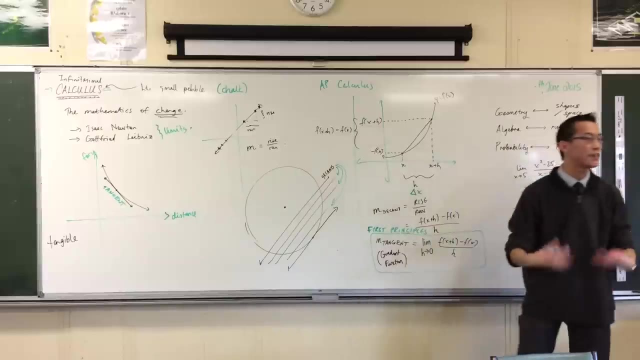 So, rather than this thing which has a gradient, Okay, This thing over here is going to be a function. It changes Right. So it's actually called the gradient of the tangent Function, Because the gradient is going to take on different values depending on where you look. 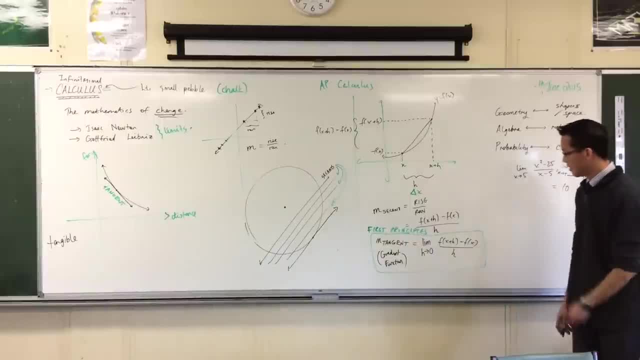 Depending on what value of x you look at. Okay Now, in the same way he said: look this, rise over run business rise over run. it's not working Because there's not really a run, Not really a run. 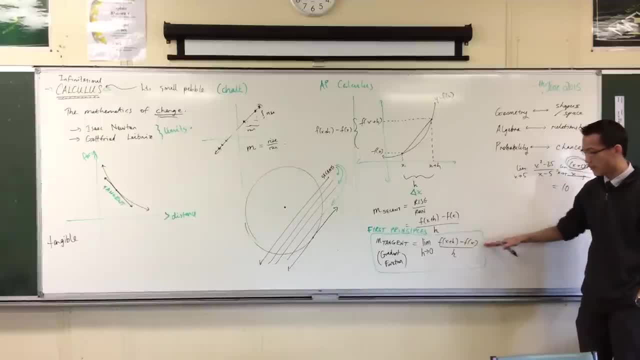 Okay. So they said: look, this is just the change in y divided by the change in x. That's all that's really happening, Right? So you guys know the symbol in science, right for change, is a delta.